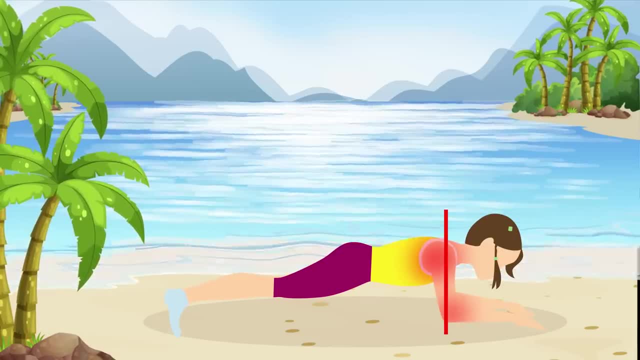 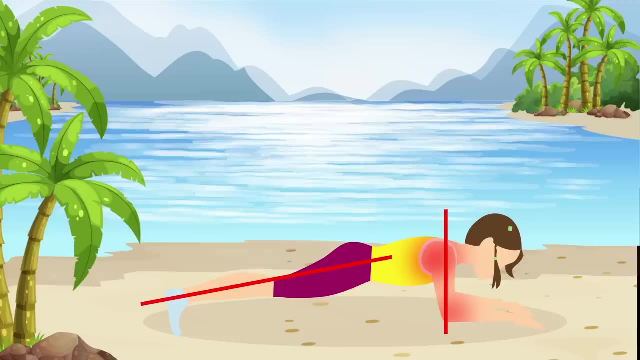 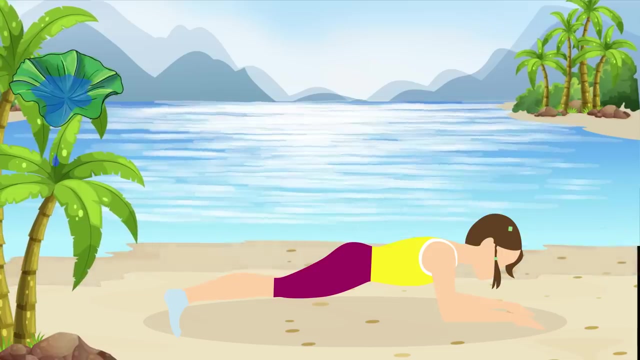 Start by getting into a push-up position. Now place your forearms on the ground so that your elbows are on the ground. Your elbows are right below your shoulders. Make sure that your body forms a straight line from head to toe, And that's it. You're planking. We'll put 30 seconds on the clock. Go. 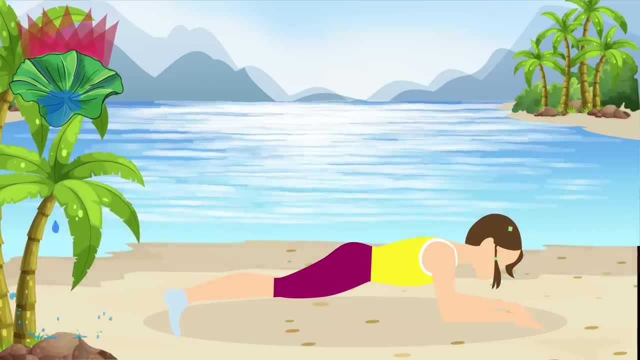 The plank is actually one of the rare exercises that not only strengthen your core but also work your entire body. It can be pretty difficult to hold, but controlling your breathing is a nice way to keep your body in shape, So let's do it. 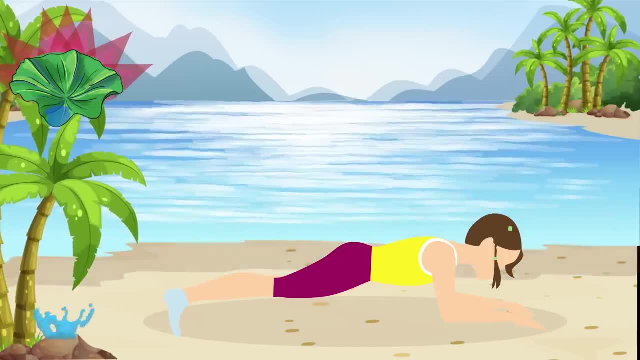 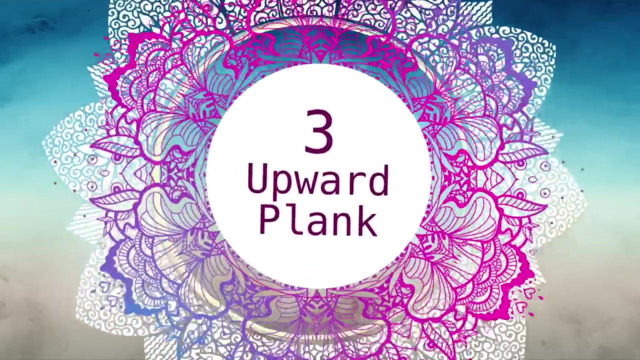 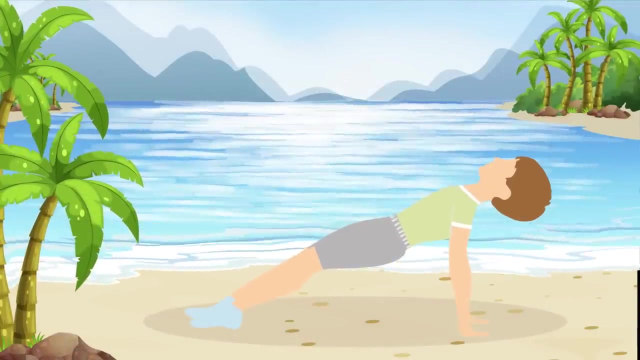 This little trick to make this exercise a little easier. Five, four, three, two, one, Well done. Pose number three: upward plank. While we're still planking, let's try another type. This one's called an upward plank. Sit on the ground with your legs straight in front of you and your feet straight in front of you. 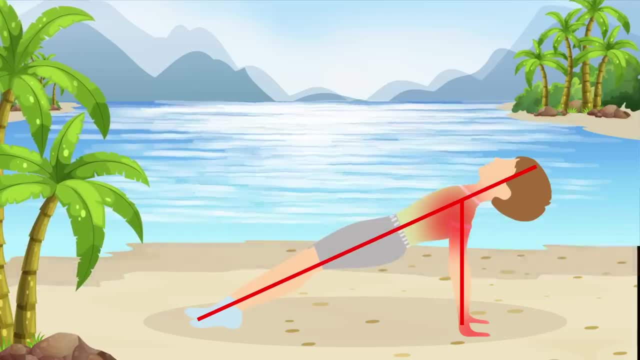 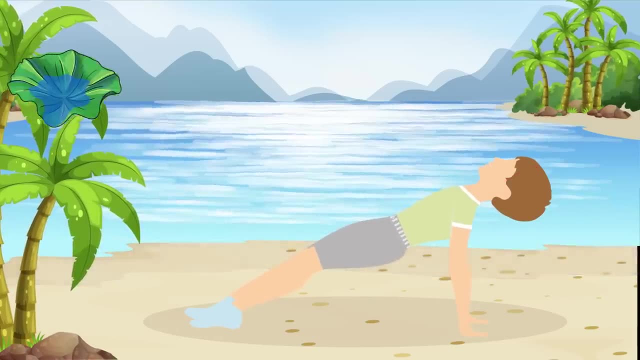 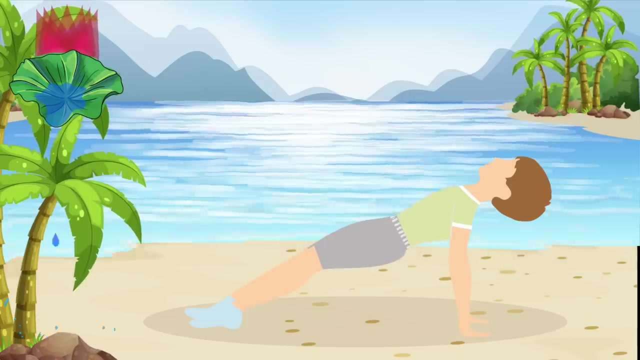 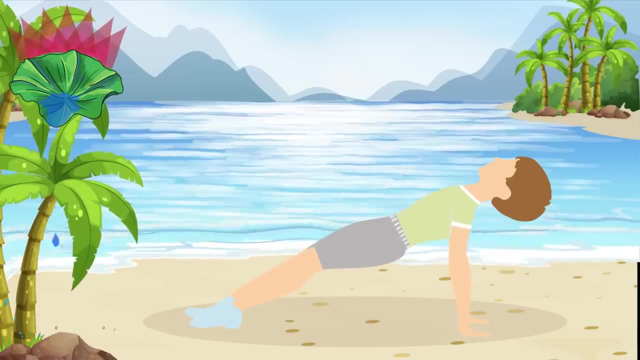 Pose number three: upward plank you and your hands behind you, Then lift your hips while keeping your toes pressed to the floor. All clear, Great, Your 30 seconds starts now. The upward plank pose stretches your upper body, improves your balance and strengthens 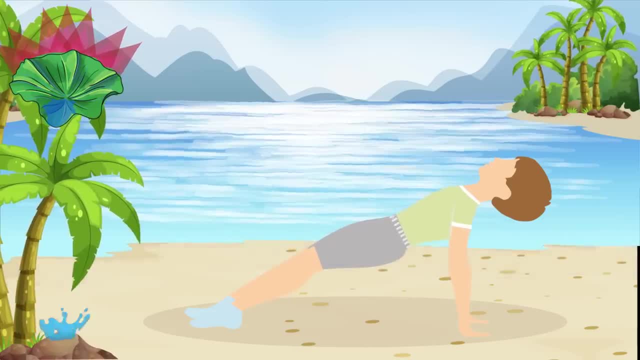 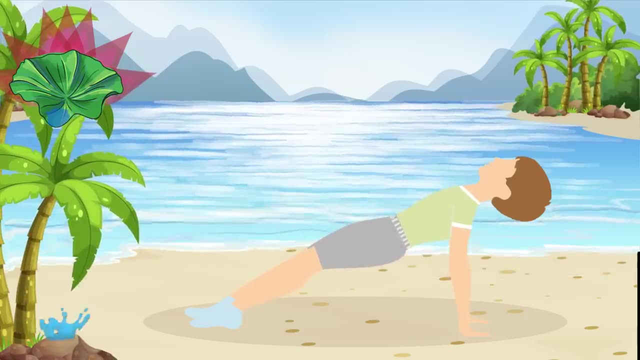 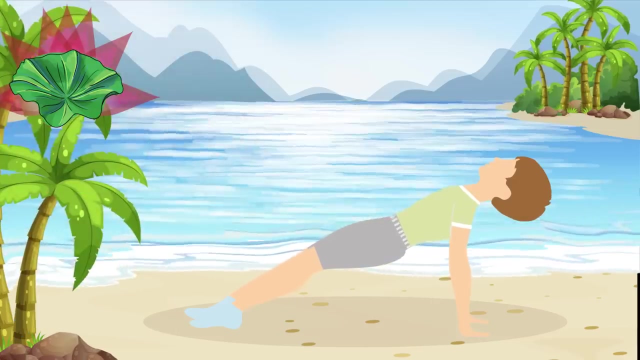 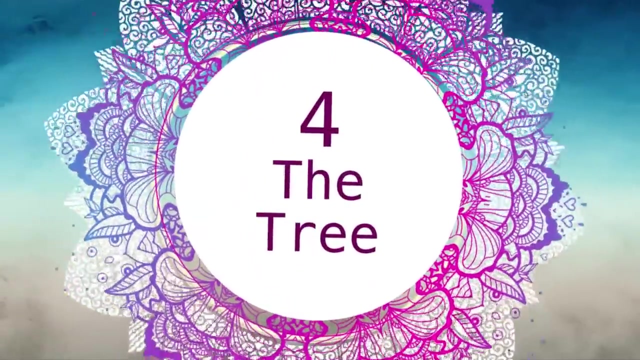 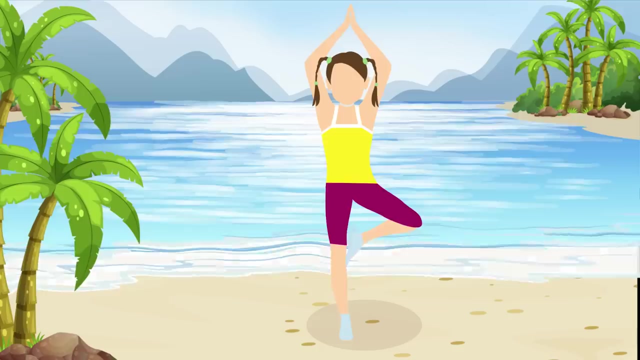 your arms, legs, glutes and core, Just like with the regular plank, control your breathing to make it easier. Five more seconds, Bravo. Pose number four: The tree. To get in the tree pose, stand tall. Stand tall with your feet together. Slowly lift your right knee up, grab it and place. 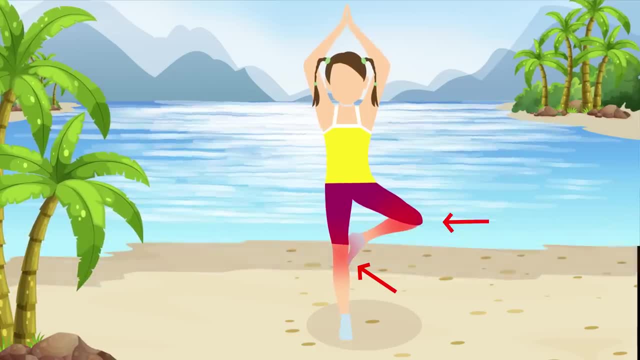 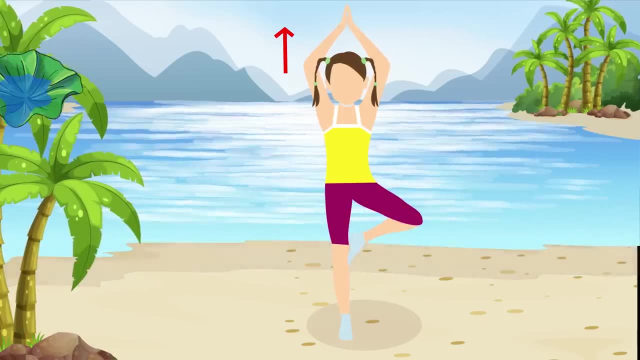 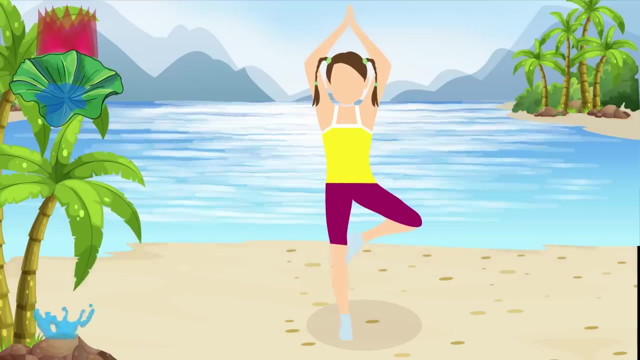 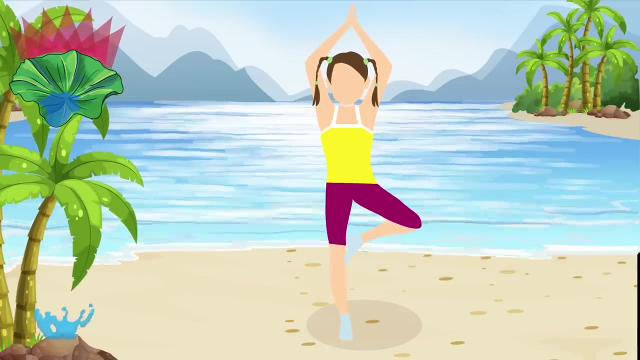 your right foot on the inner thigh of your left leg, close to your groin. Now lift your arms up to the sky with your palms together. Let's begin with your right leg raised for 30 seconds. If you're completely new to the world of yoga, practicing the tree. 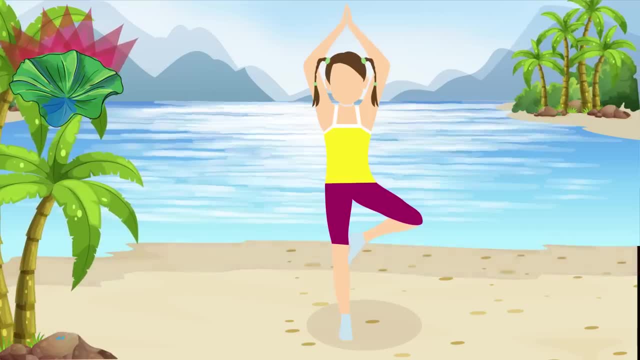 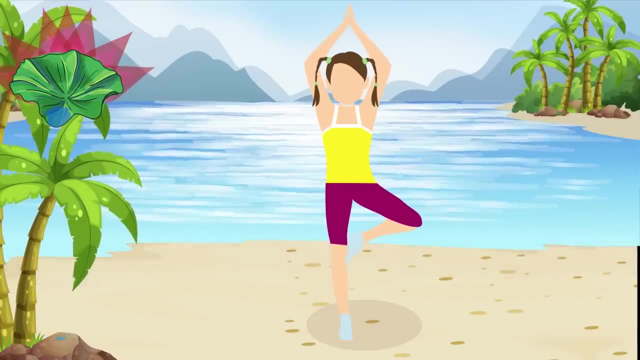 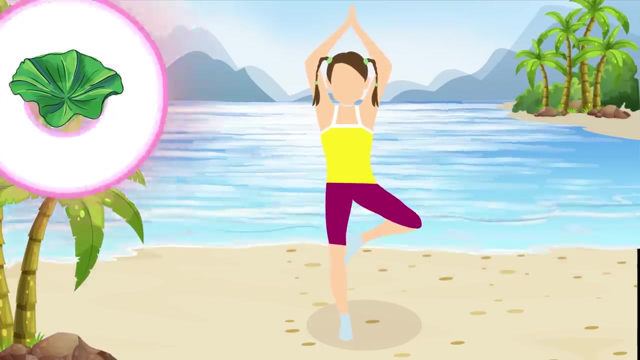 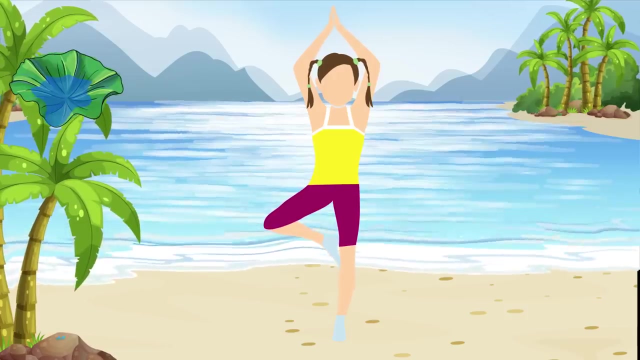 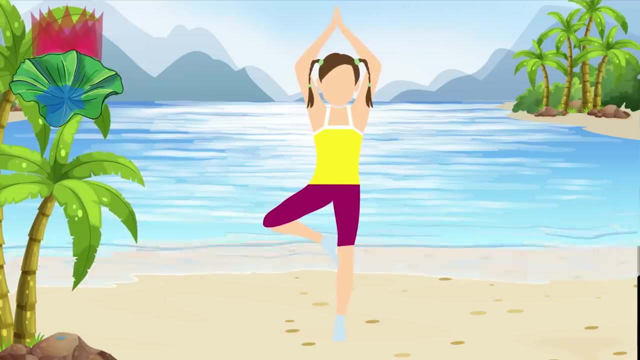 pose is definitely a great starting point. It improves your balance and teaches you how to breathe correctly. You're doing great. Keep it up And amazing. Now let's do the same thing with your left knee raised. You're doing great. Keep it up And amazing. 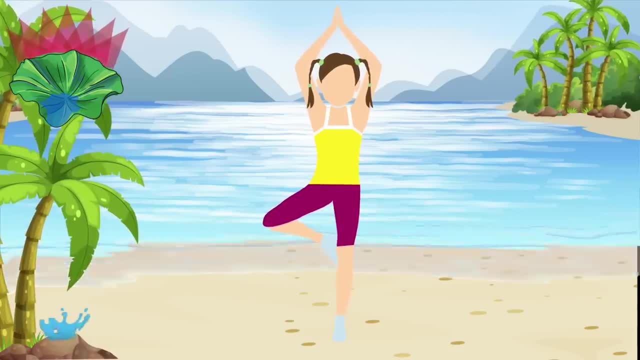 Tree pose also strengthens and tones the calves ankles and inner thighs, So doing this exercise regularly will leave you with some very nice looking legs. As an added bonus, it also does a lot for your core. Three, two, one done. 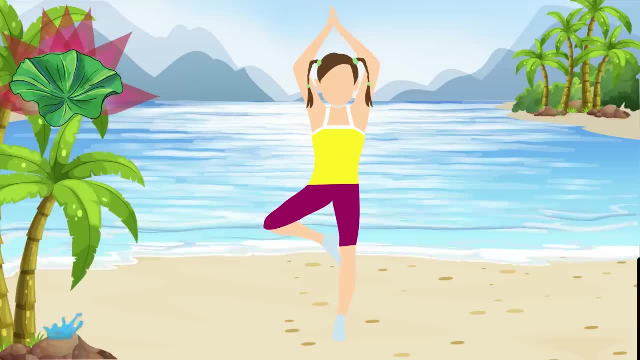 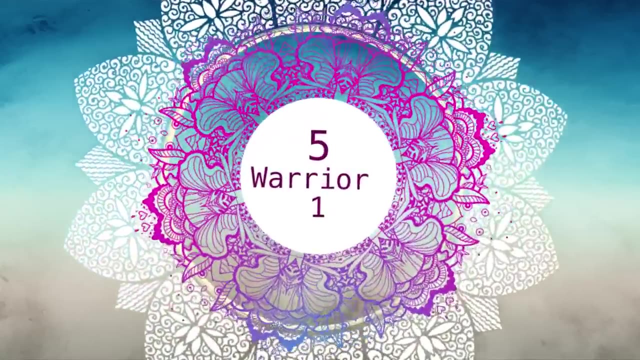 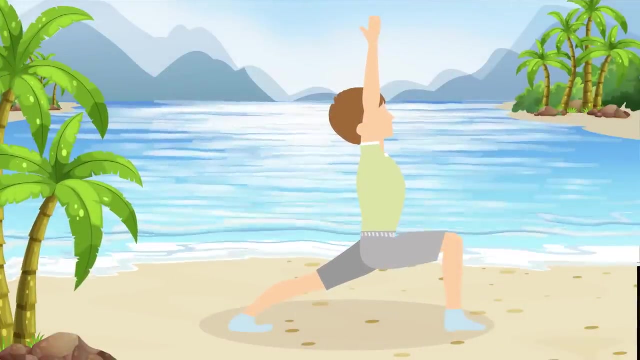 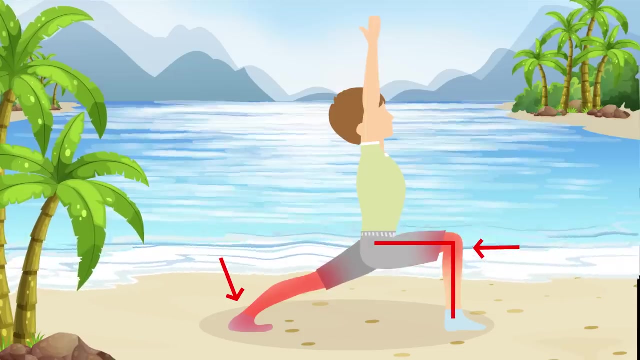 Three, two, one done. Pose number five, warrior one: Take a really wide stance and rotate your hips so that your right leg is in front of you and your left leg is behind you. Bend your right knee so that your shin forms a. 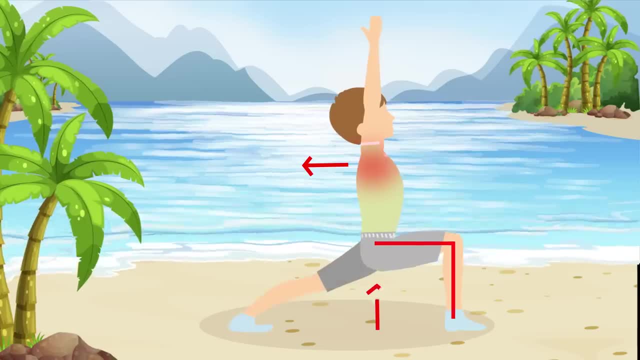 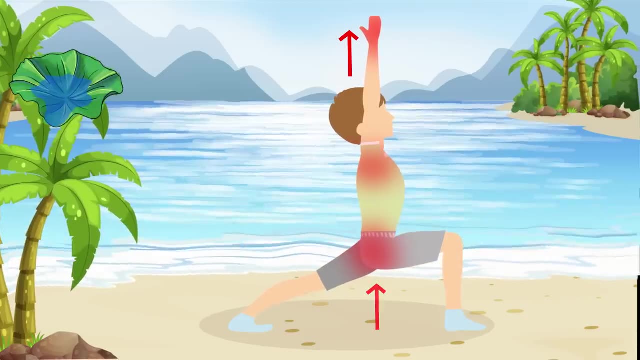 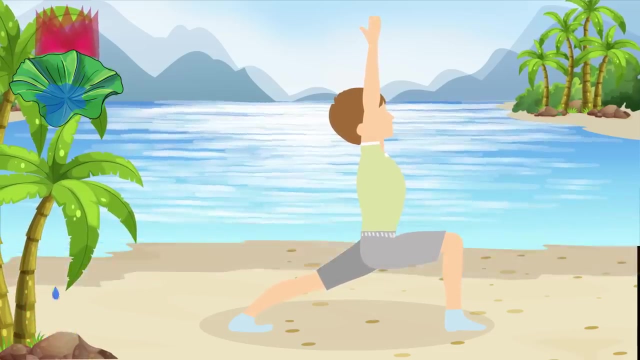 straight vertical line. Roll your shoulders back, lift your chest and reach your arms with your palms together. Let's do 30 seconds on the right foot. Three, two, one done. Warrior. one stance is one of the main poses in many yoga practices. It's essential for 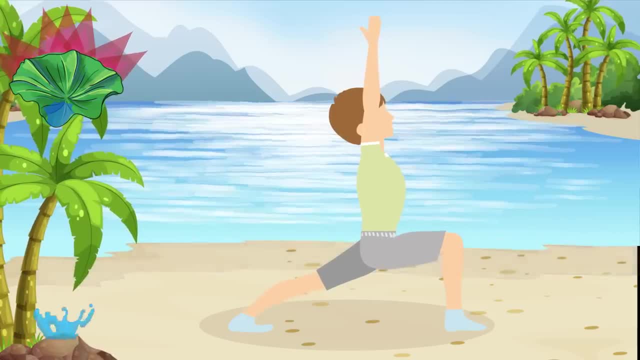 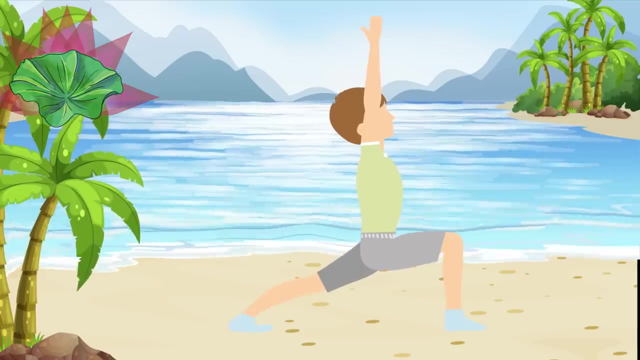 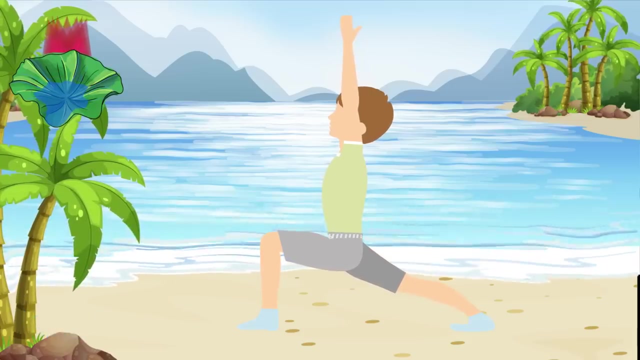 improving the strength of the core and the entire lower body. While you're doing it, be sure to breathe calmly. You're doing great, Keep it up And amazing Tree pose. And now change it up to your left leg. 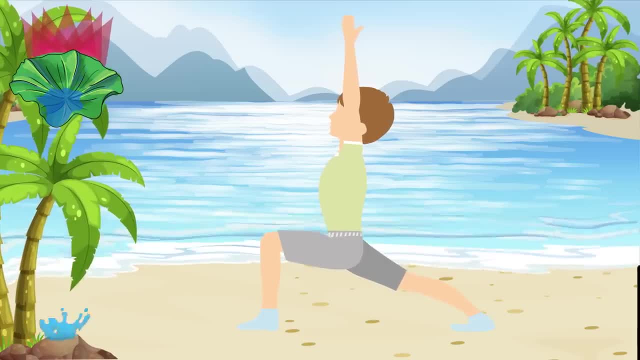 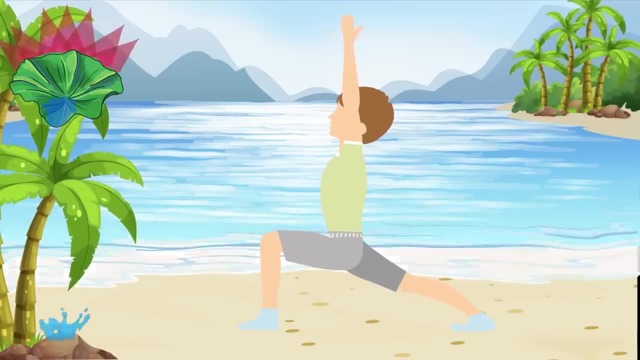 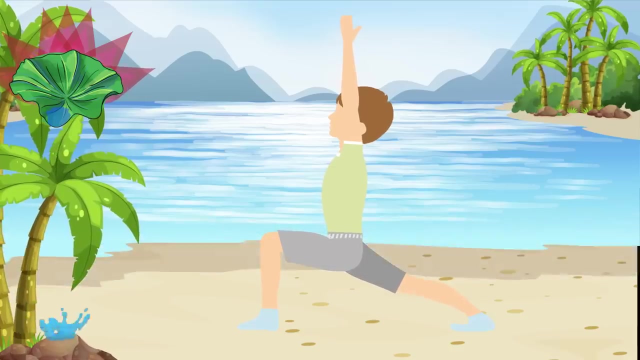 Among other things. Warrior One also gives a good stretch to your chest, lungs, shoulders, hips, thighs, and the list goes on. Try not to tip your pelvis forward, as it can put too much pressure on your lower back. We're almost done and that's it for Warrior One. 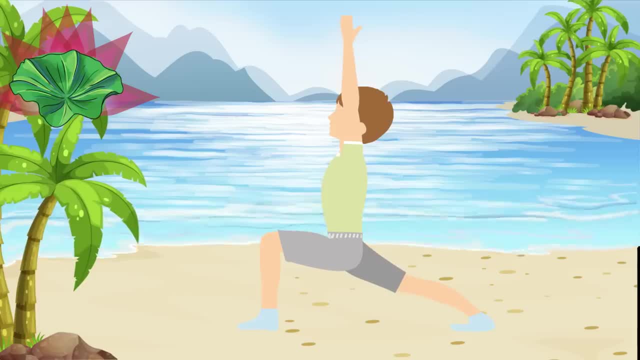 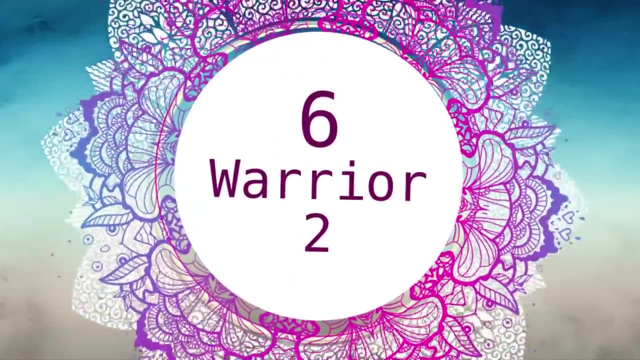 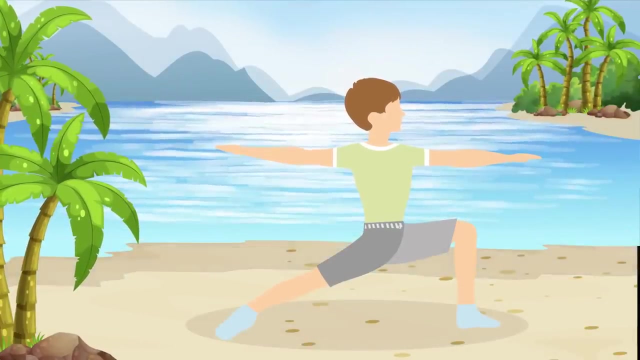 Now get ready for Warrior Stance Two, Pose Number Six: Warrior Two: Like Warrior One, Stand with your feet about one leg length apart, but don't square your hips this time. Turn your right foot out and bend that knee at a 45-degree angle. 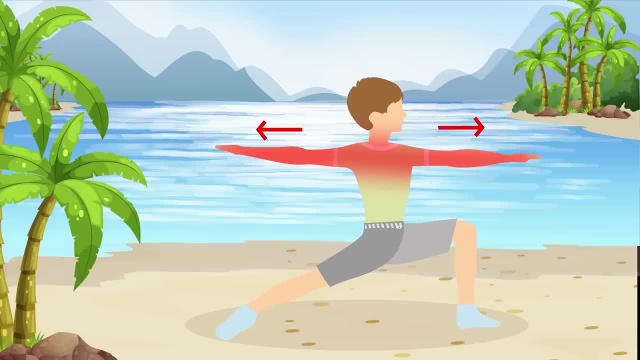 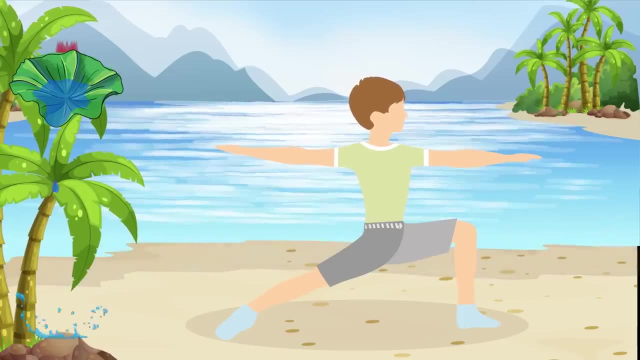 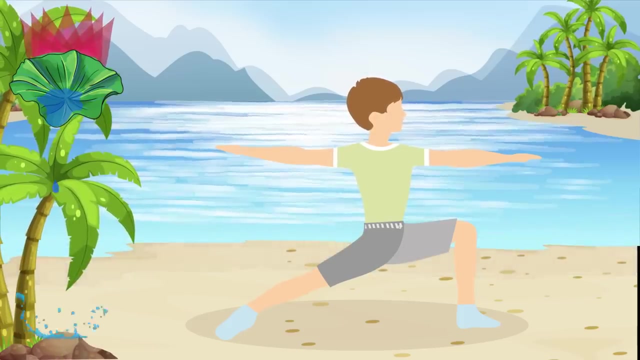 Now stretch your arms out to the sides and gaze over with your right hand. Let's do half a minute on the right side. Warrior Two: stretches your hips, Bend your knees and raise your hips and inner thighs, while improving your balance tenfold. 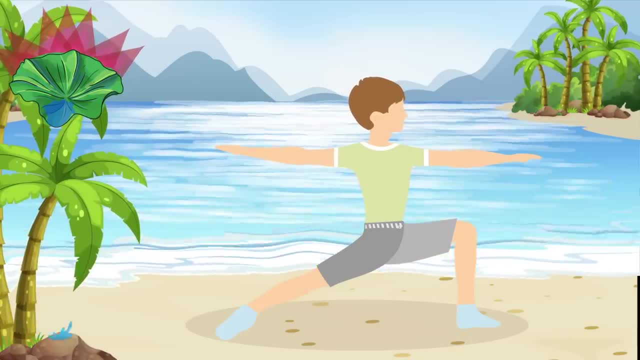 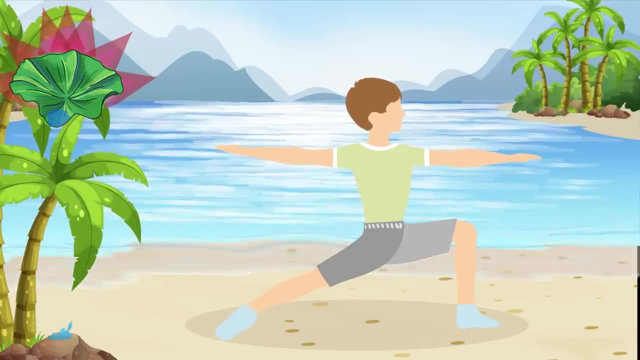 An important一個 important- thing to remember is to not bend your knees too high If you have any kind of neck problems. don't turn your head to look over your hand though. Just look straight ahead. Okay, Now let's do the left side. 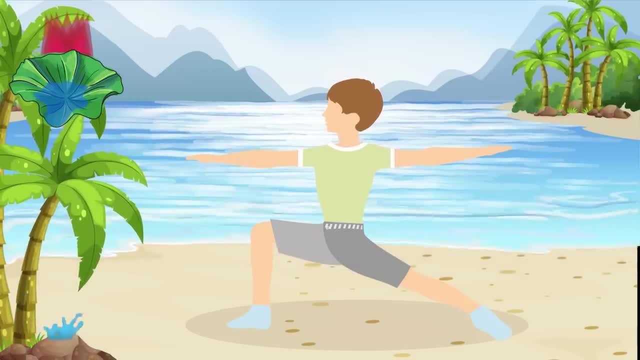 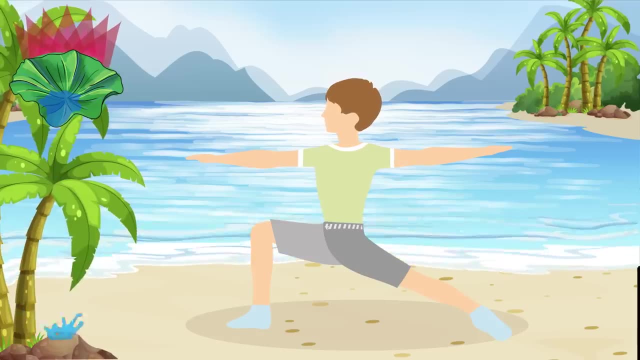 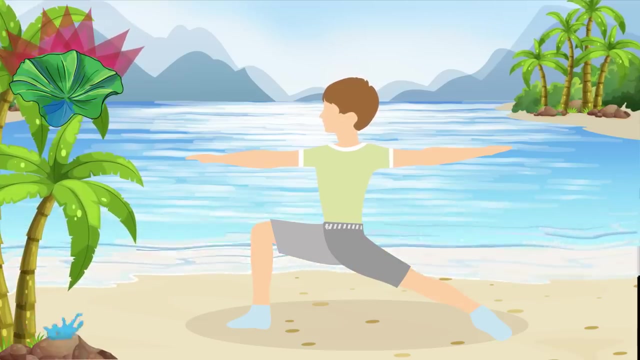 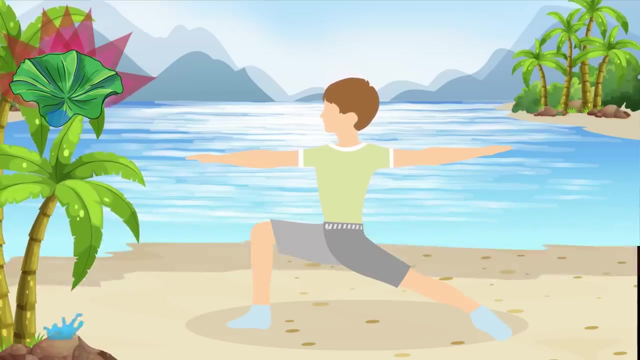 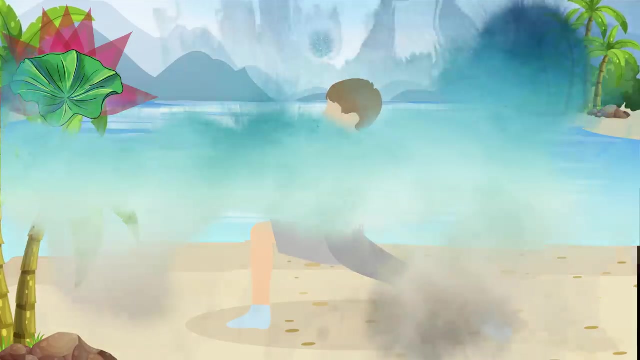 Okay, Now let's do the left side, Okay. Warrior 2 can also help improve digestion and relieve backaches, Not to mention it significantly increases your stamina, making you stronger both physically and mentally. Just a couple more seconds and done. 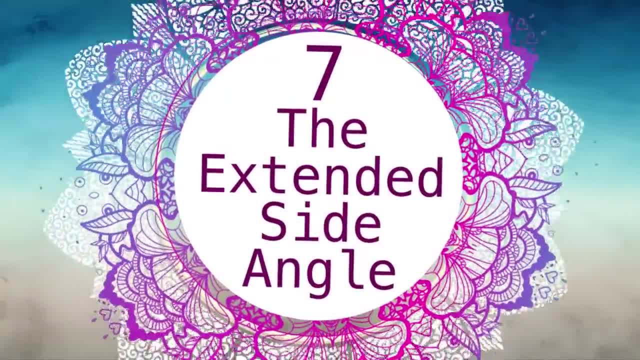 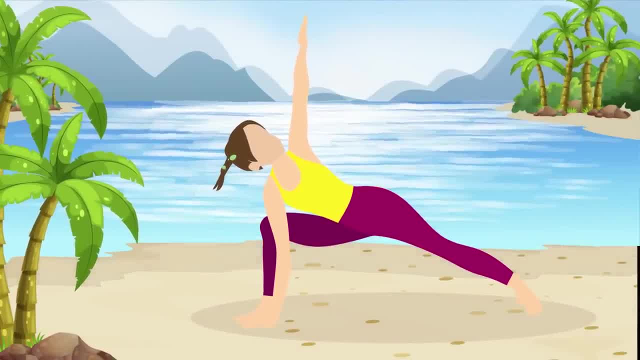 Pose number seven: the extended side angle. Start by getting into Warrior 2, only, instead of stretching your arms out to the sides, bend your body to place your right hand on the floor next to your right foot, Then stretch your left hand up towards the ceiling, keeping a straight line from the 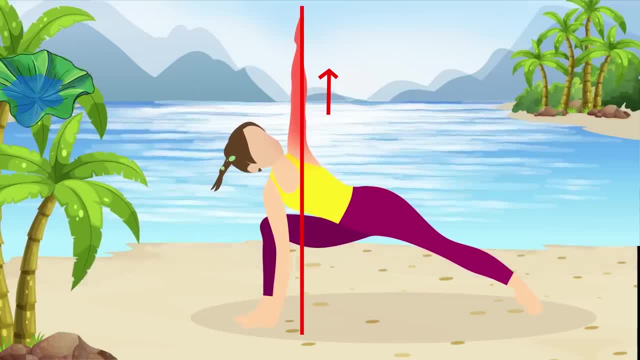 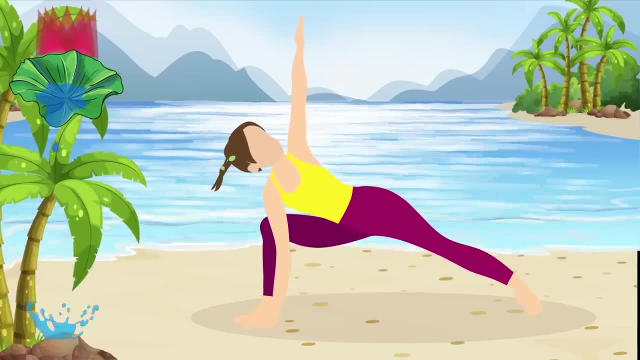 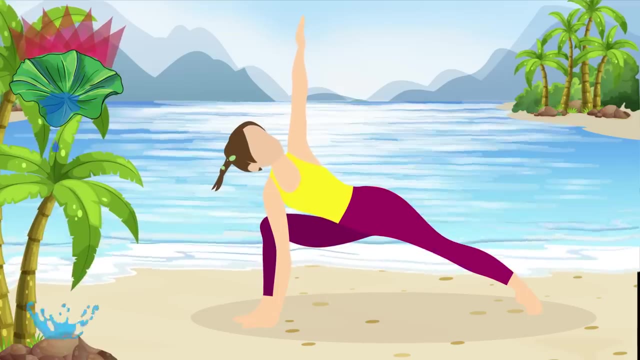 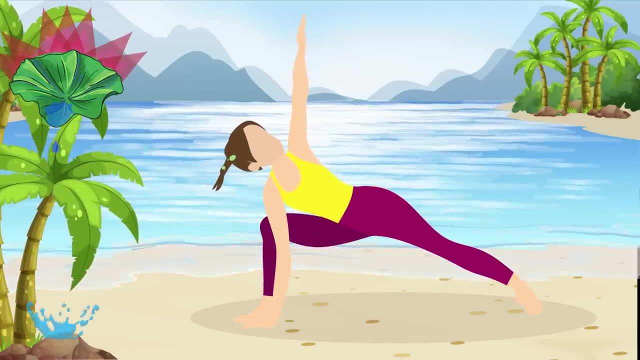 right hand to the left. As always, let's begin with the right side. This particular pose is designed to target the sides of the torso and strengthen the legs, hips, hamstrings, calves, shoulders, chest and spine, So basically your whole body. 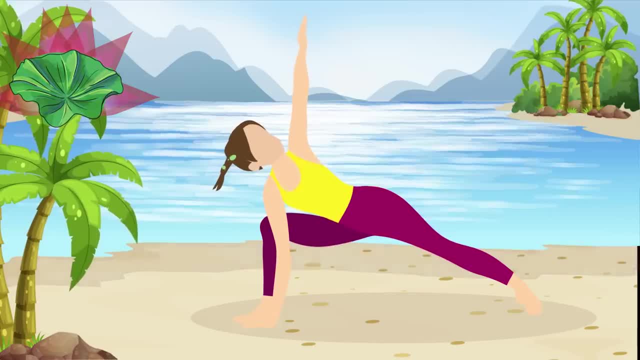 Not bad, right. And now time to switch to your left side. Pose number seven: the extended side angle. Start by getting into Warrior 2, only, instead of stretching your arms out to the sides, bend your body to place your right hand on the floor next to your right foot. 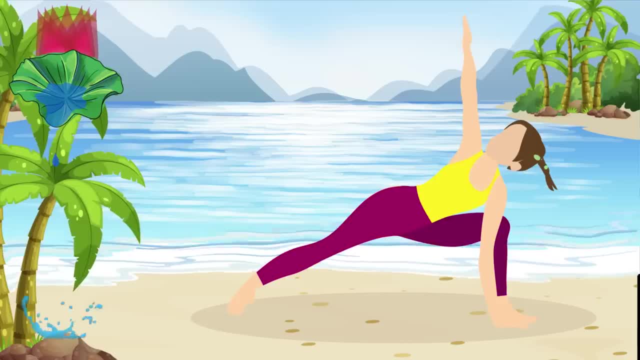 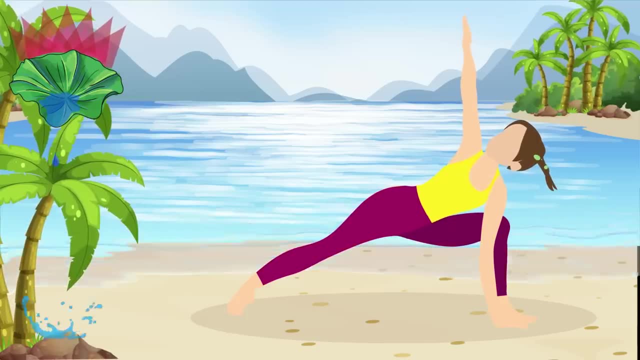 Then stretch your left hand up towards the ceiling, keeping a straight line from the left side. The extended side angle pose also opens up the lungs, improves digestion and helps relieve stress. Oh, and it can sharpen your mind too. Try to focus on exactly what each part of your body is doing during the pose. 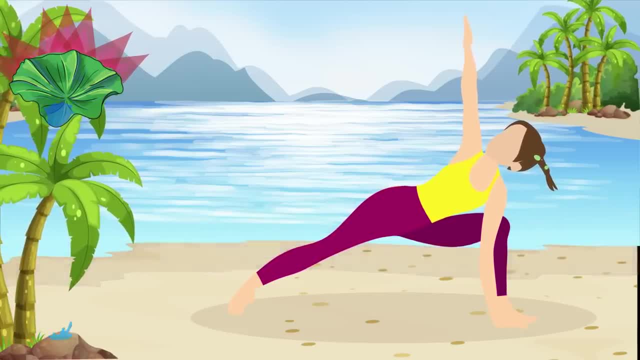 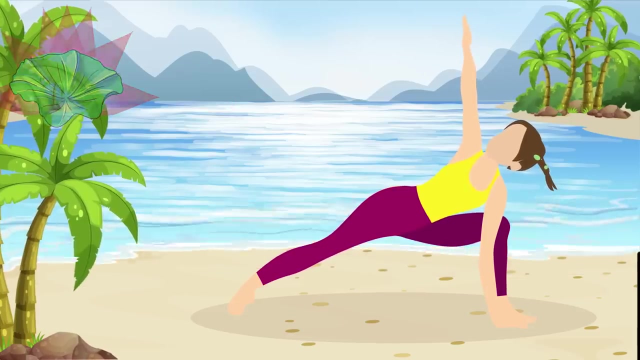 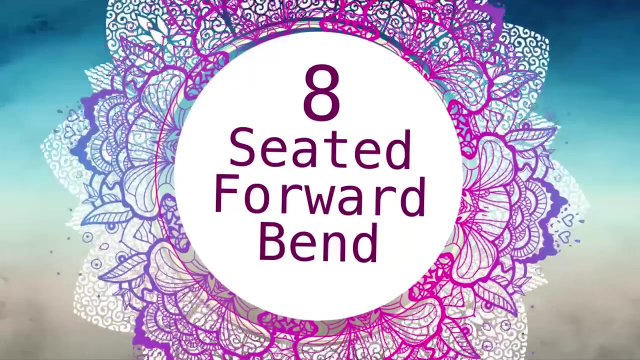 Doing this regularly will make all of your problems with concentration disappear. Pose number five: the extended side- angle Side. Samsa, And that's it for this pose. Take a deep breath and let's move on to the next one. Pose number eight: Seated forward bend. 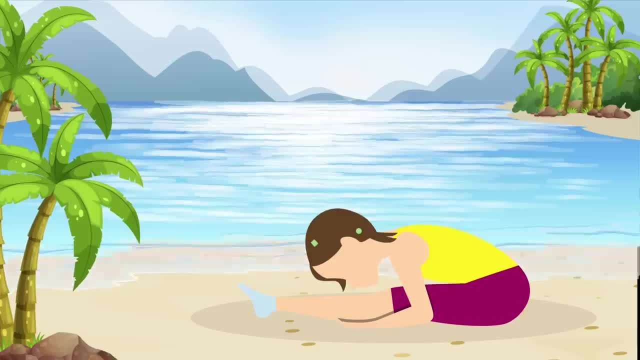 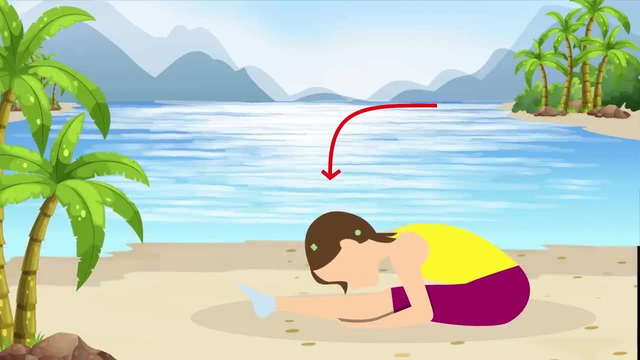 Let's get back down on the floor, shall we Sit down with your legs pulled together, straight out in front of you? Now start to lean forward from your waist, reaching for your toes. Once you've reached your limit as far as stretching goes, hold it for the next 30 seconds. 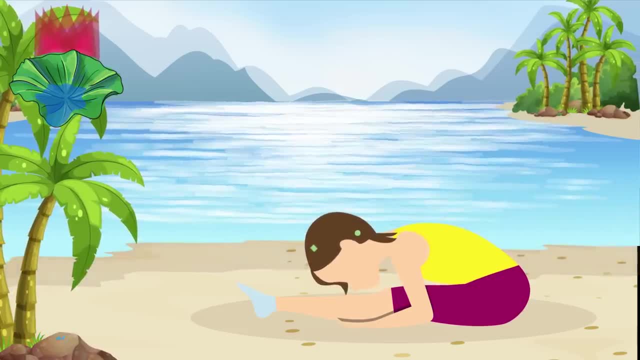 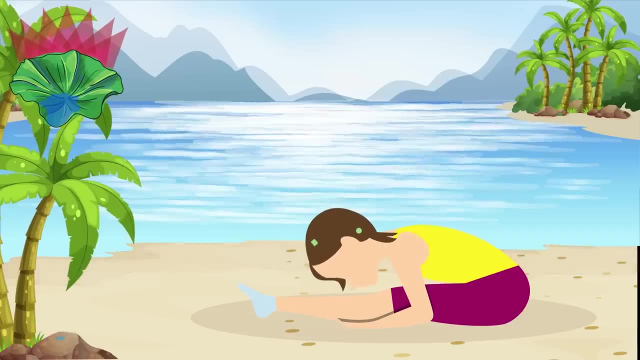 You can probably feel it right about now, but this pose is awesome for stretching your lower and upper back, as well as your hamstrings. It opens up the entire body, teaches you to breathe when you're in an uncomfortable position, helps with headaches and anxiety and reduces fatigue. 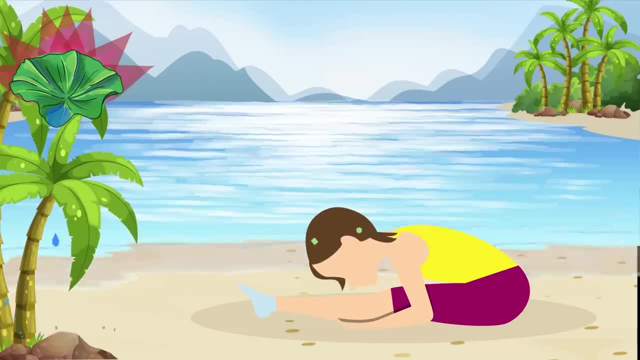 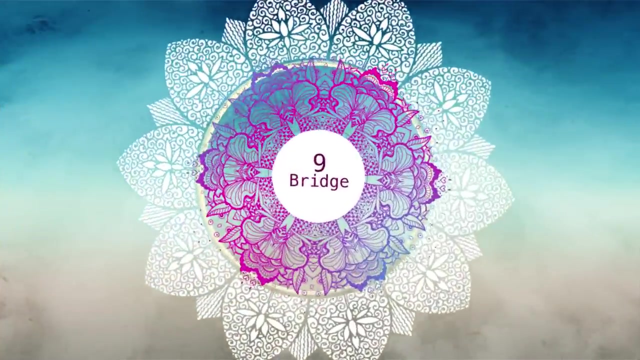 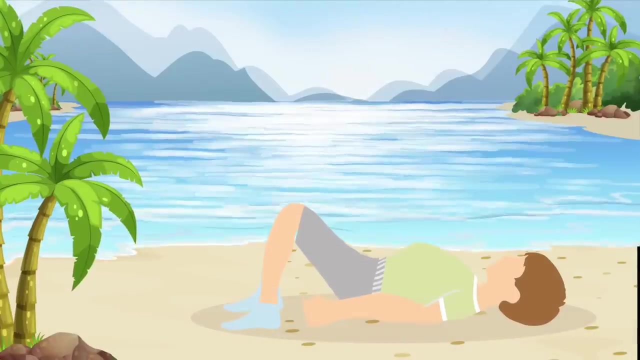 Just make sure to keep your back straight and do the pose correctly. Hold it a little more and nailed it. Pose number nine, Bridge: Lie on your back with your knees bent up, Lift your hips up towards the ceiling and hold this position. 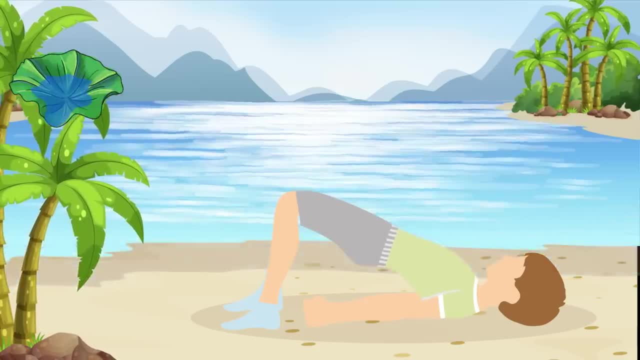 Yep, it's pretty straightforward. Your time starts now. The bridge is yet another essential pose for beginners. It manages to stretch both the front and the back of the body. It also improves blood circulation and digestion, helps relieve stress and opens the lungs and thyroid. 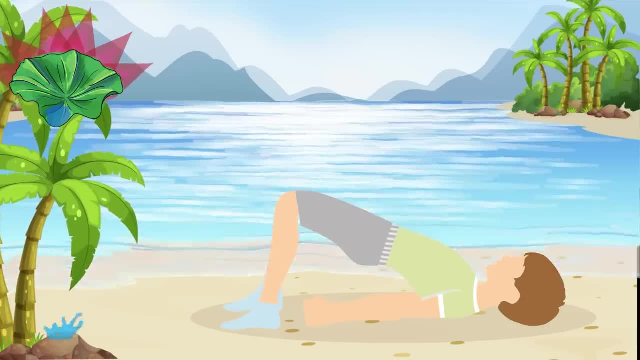 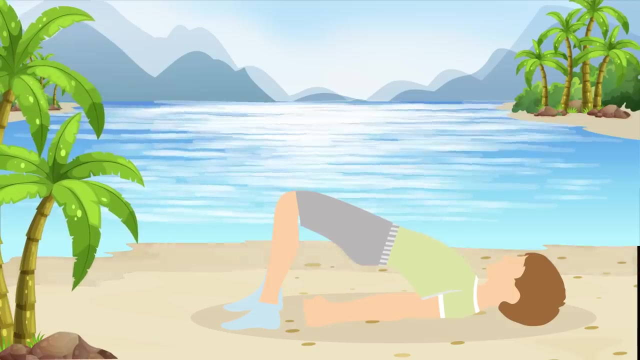 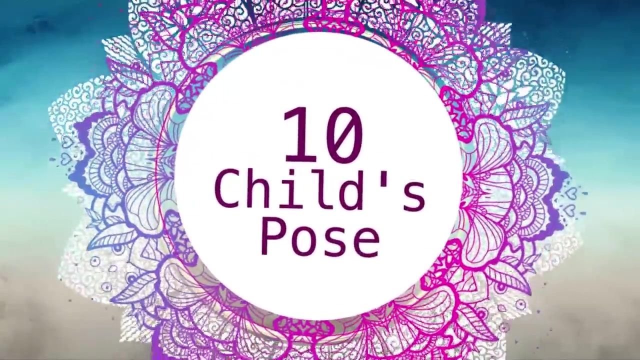 Not that many exercises can do that right. Hold it and done. Keep up the energy. The next exercise is right around the corner. Pose number ten: Child's pose. Start child's pose by sitting on your knees on the mat. 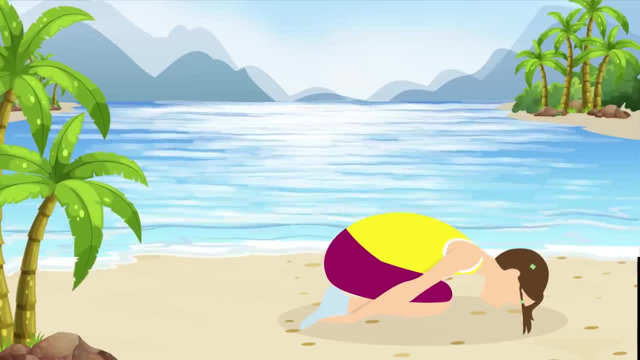 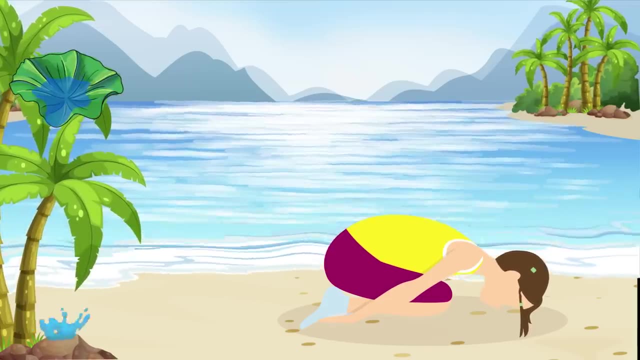 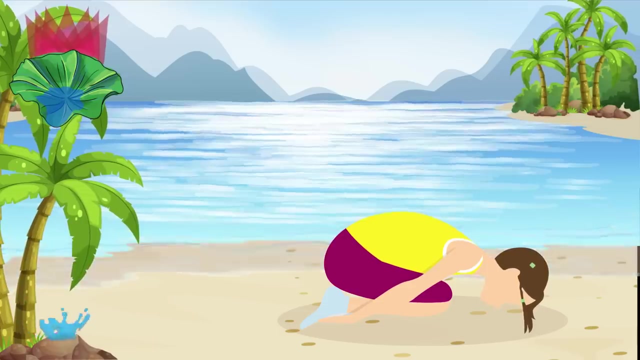 Then lower your head to the floor with your hands reaching forward or rested at your sides. Now just relax for the next 30 seconds, Hold it and done. Child's pose is the best resting pose for any stress and tension relief. 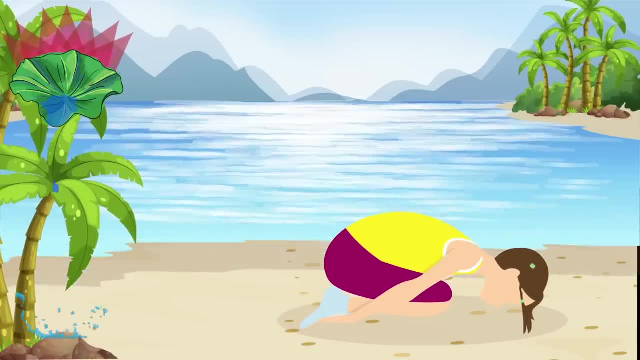 It's also good to do it in between difficult exercises to calm down your body and mind. Plus, it improves your digestion, relieves back and neck pain and stretches your hips, thighs and ankles. Hold it and done. Start child's pose by sitting on your knees on the mat. 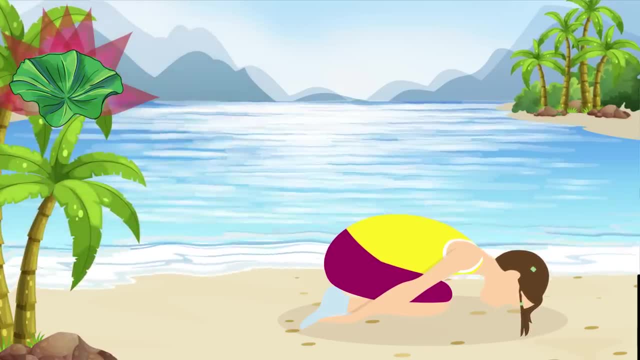 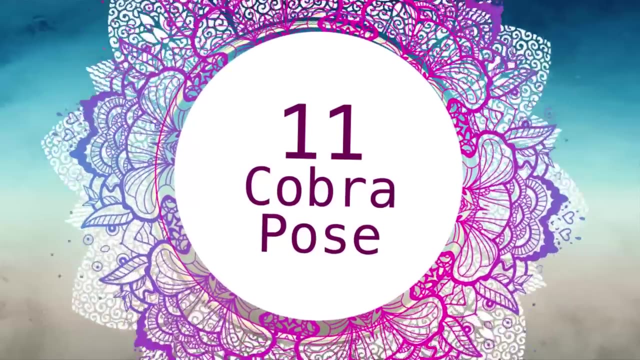 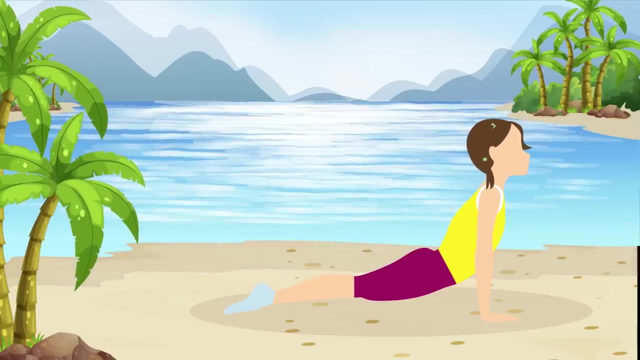 Then lower your head to the floor with your hands reaching forward or rested at your sides, Hold it and done, And time's up. Pose number eleven: Cobra pose. To get into cobra pose, start from the downward facing dog. 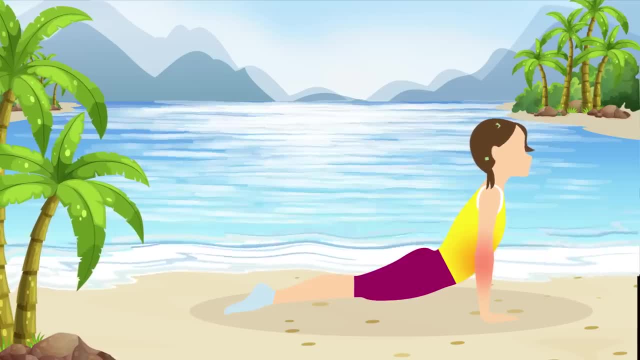 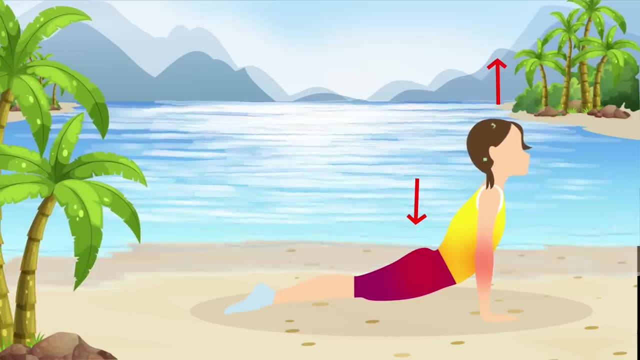 After that, come forward into a plank, bend your elbows and slowly lower your hips down to the floor. Roll your shoulders back and gently lift your upper body, Elegant and easy, Ready to hold it for the next 30 seconds. Then let's get to it. 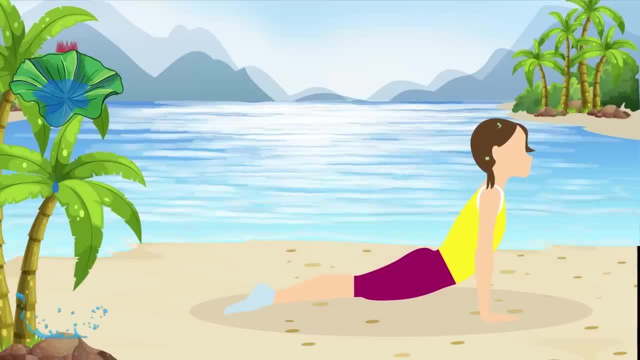 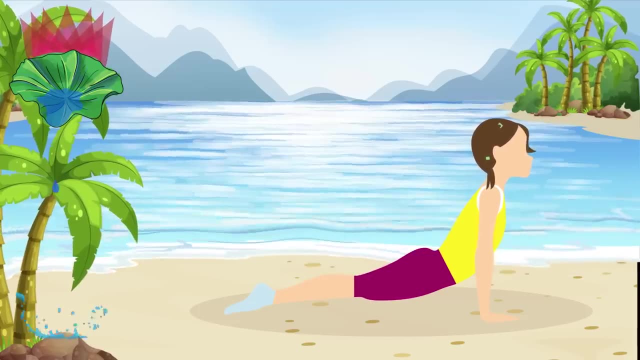 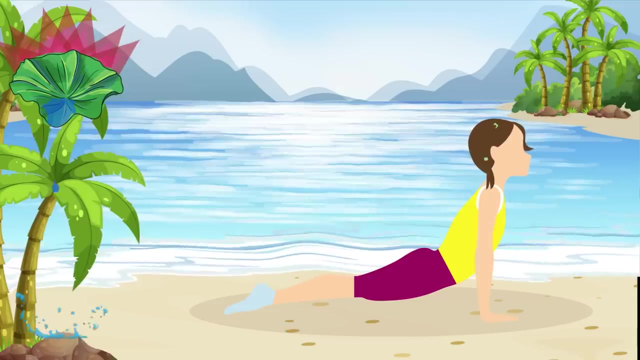 it. This pose strengthens your back and opens up your chest and shoulders. It also decreases stiffness in the lower back. Do it carefully. if you have any back injuries, In that case it's actually better to stay away from this pose until you get better. 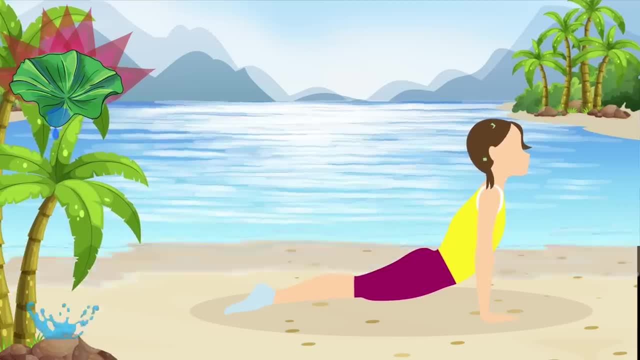 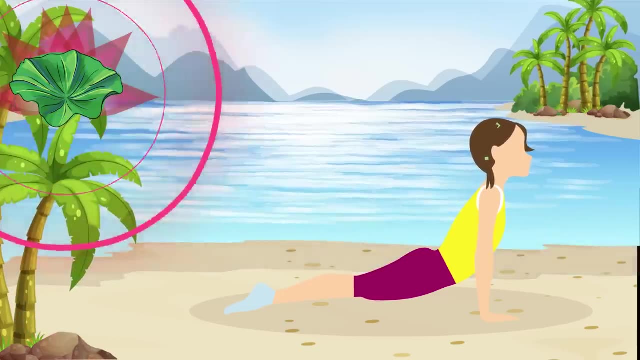 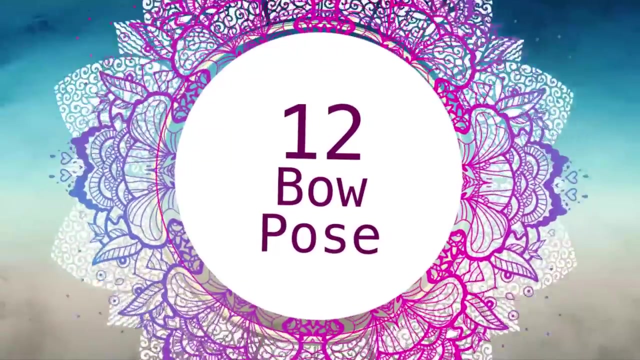 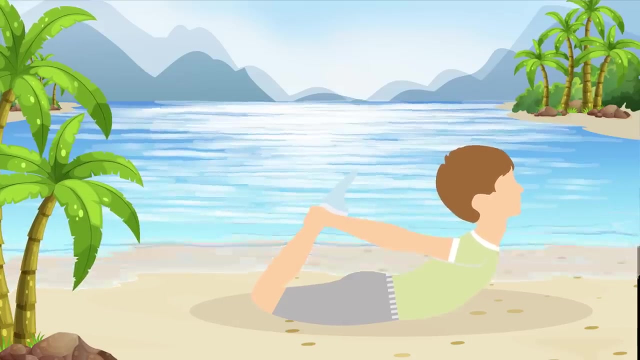 Three, two, one nice Pose number 12, bow pose. This one's not too hard, depending on your flexibility. Just lie on your stomach on the ground or mat, Bend your knees. lift your thighs up off the floor and bend your knees. This one's not too hard, depending on your flexibility, Just. 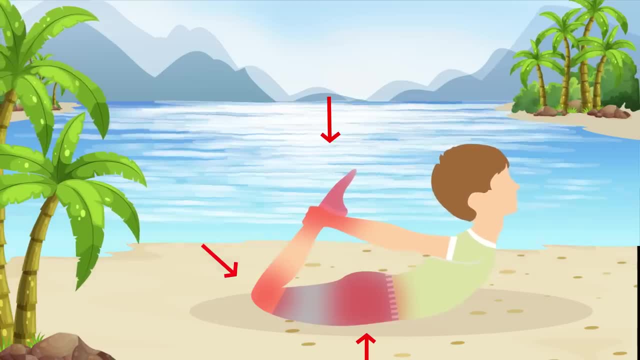 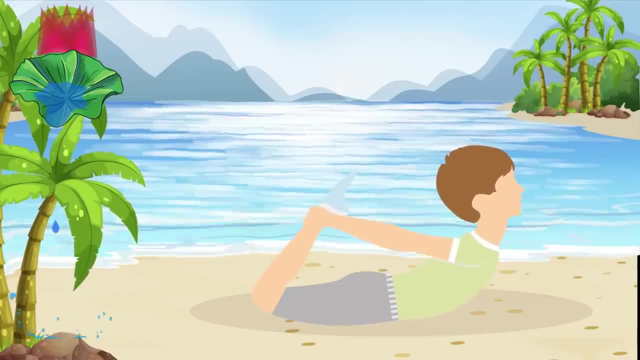 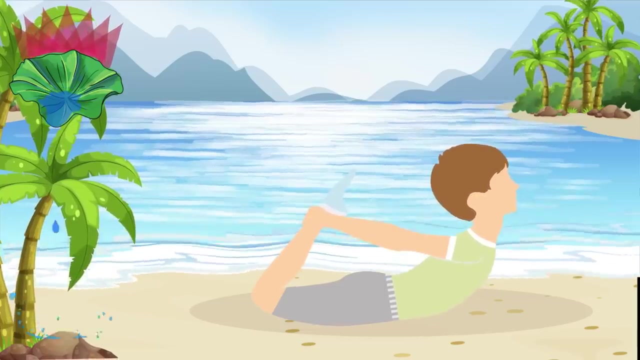 bend your knees, lift your thighs up off the floor, reach back and grab your ankles. Hold it there for half a minute. Bow pose is a miracle for stretching the whole front and back of your body, while additionally improving your posture and spinal flexibility. However, if you have 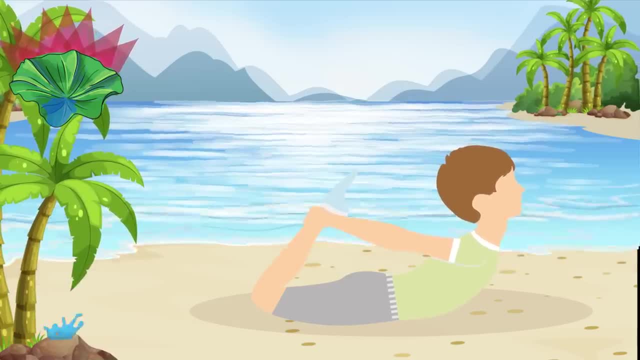 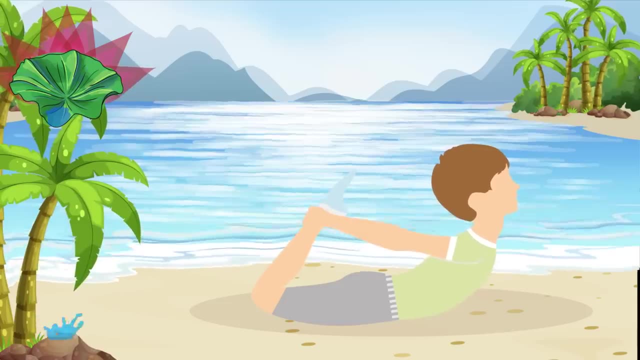 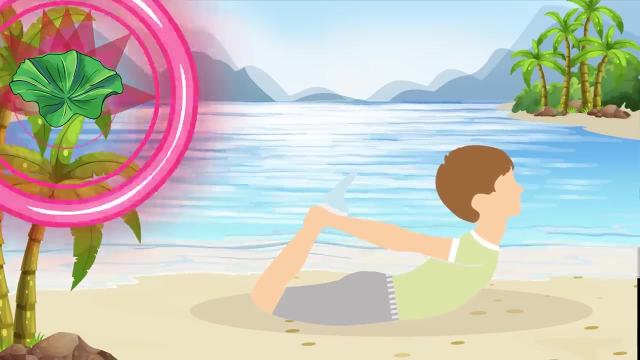 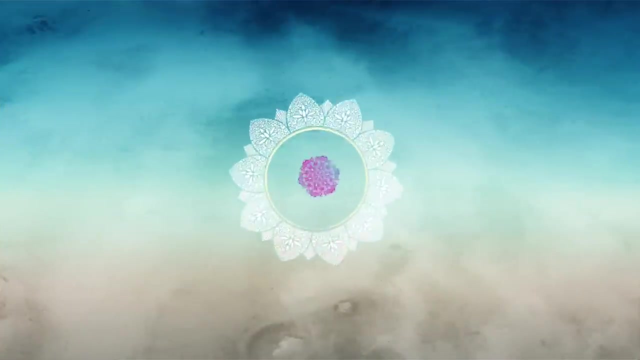 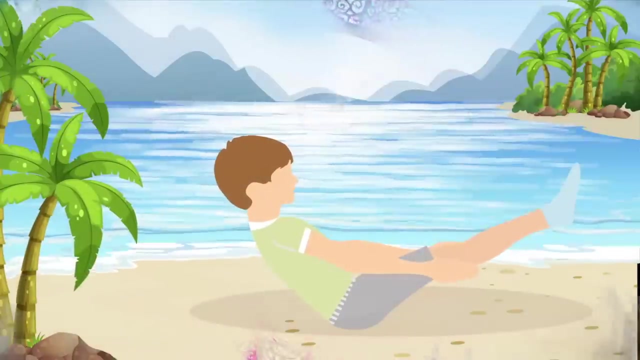 frequent migraines or insomnia, it's better to avoid this pose. The same goes for those diagnosed with high or low blood pressure. Just replace this one with a different yoga pose And wonderful. Three more exercises to go. Pose number 13,: boat pose: Start by sitting on the ground, Bend your knees, lean back. 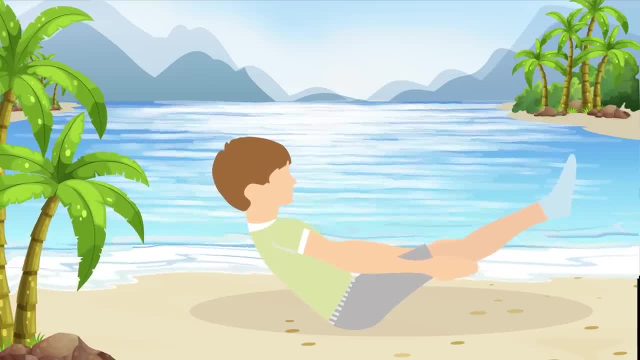 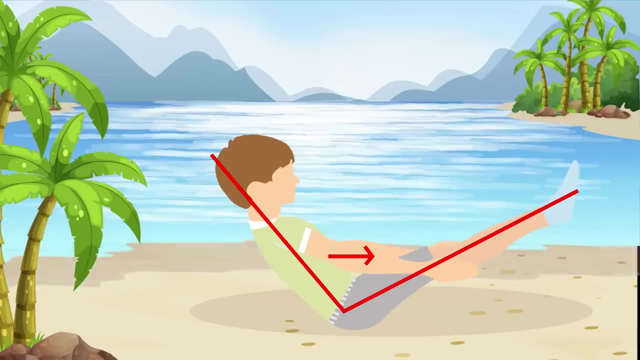 and lift your feet until your shins are parallel to the floor. If you feel comfortable with this position, extend your knees and bend your thighs. If you feel comfortable with this position, extend your arms forward. Straighten your legs so that your body makes a V-shape. There you go. 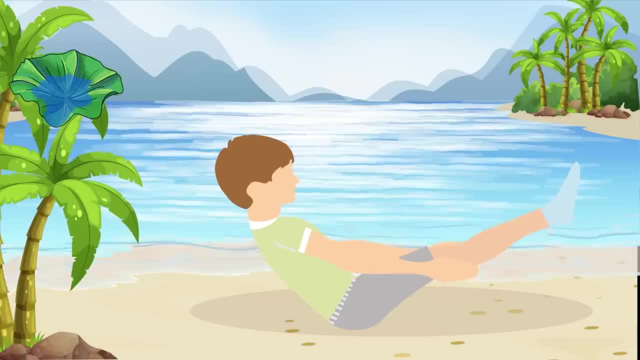 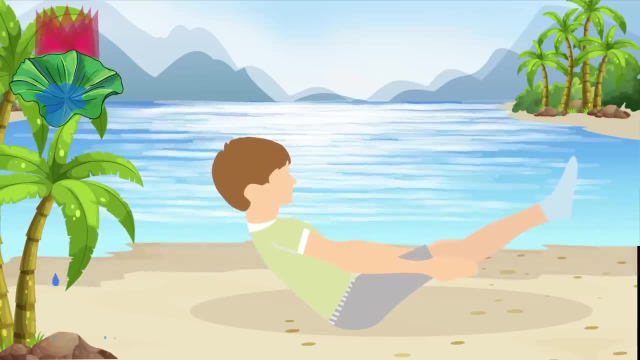 You're now a boat, Be one for the next 30 seconds. Boat pose is a huge stress reliever. It also improves digestion, stimulates the kidneys, thyroid and intestines and strengthens the thighs and lower back. If you're a lady and it's. 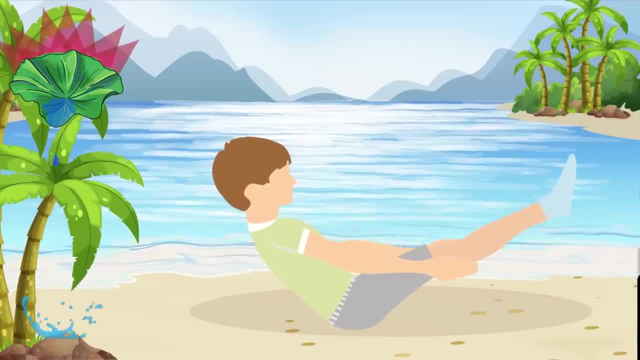 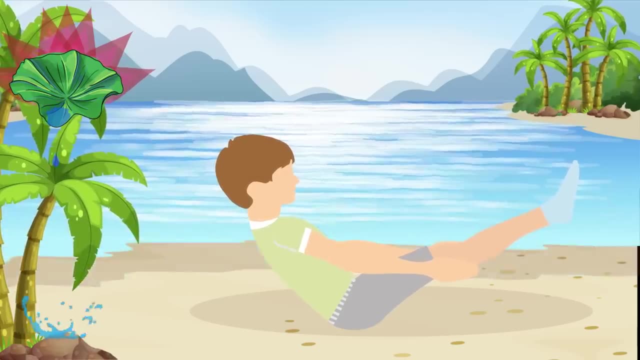 that time of the month you're better off skipping on this pose, since it won't be very beneficial for you to do it. If you're a lady and it's that time of the month, you're better off skipping on this during your period. It's also not advisable to do it regularly if you suffer from asthma or diarrhea. 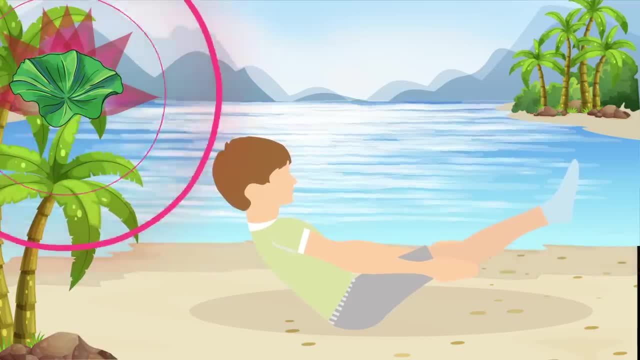 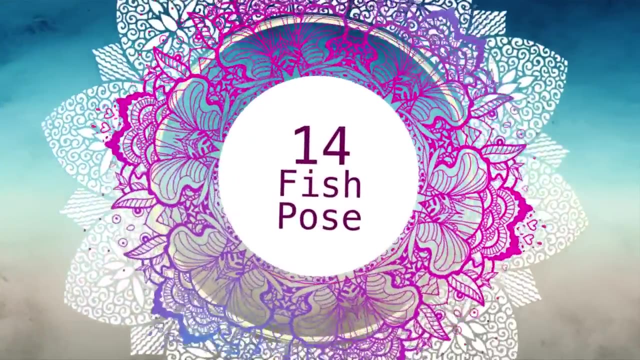 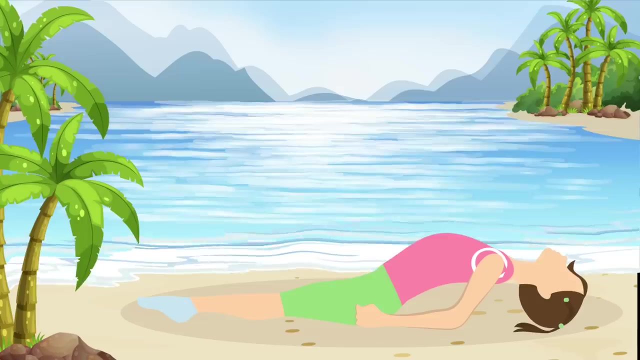 Three more seconds and stop. You're doing great, Keep it up. Pose number 14, fish pose. For this one, start off by lying on your back, keeping your feet on the floor and your knees bent. Then lift your arms up and bend your knees If you're a lady and it's that time of the month. 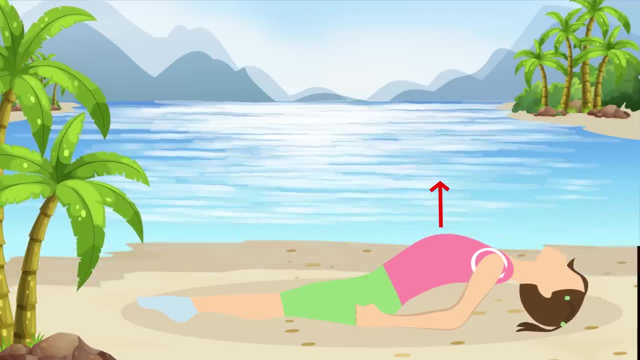 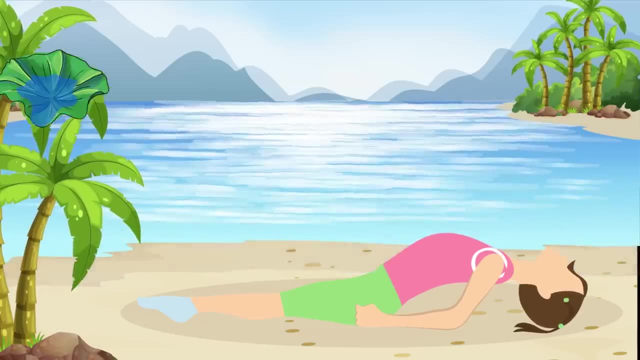 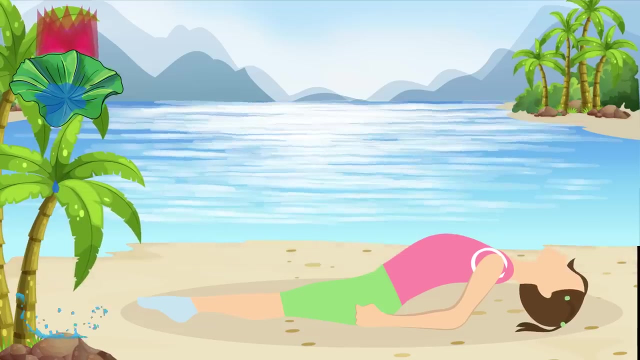 keep your upper body while sliding your hands under your butt. Keep your forearms and elbows close to the sides of your body and lift your upper back off the floor. Your 30 seconds begin right now. This pose strengthens your hamstrings and lower back. It also opens up your hips and